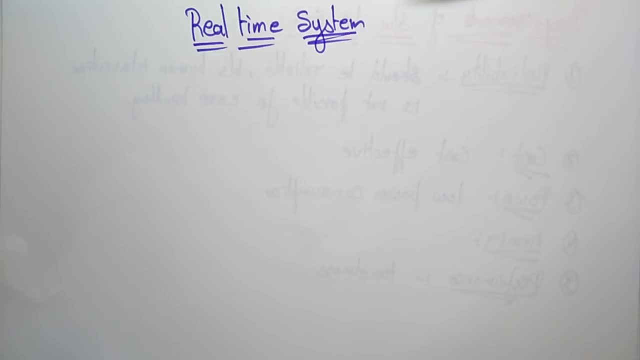 Students, welcome back. Coming to the next topic in the subject, embedded systems, was real-time systems. So this real-time system is one of the important concepts while you are designing the embedded system. So, whatever the system you are going to design by means the microcontrollers or the chips you are designing, So it's a combination of hardware and the software. So that software that you are going to develop is make sure that you are using the real-time system. 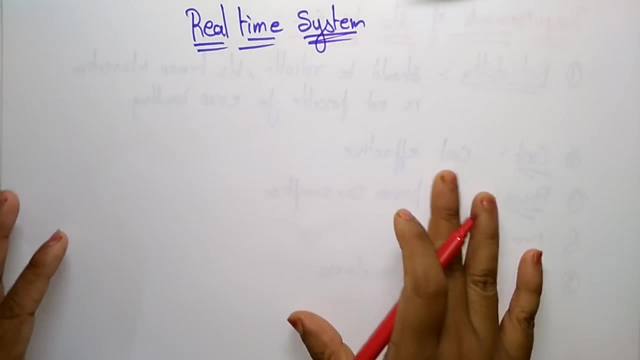 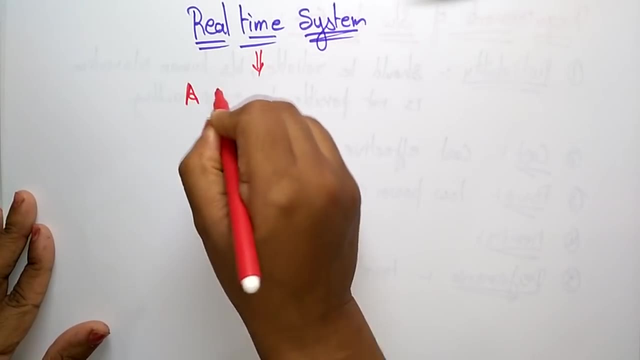 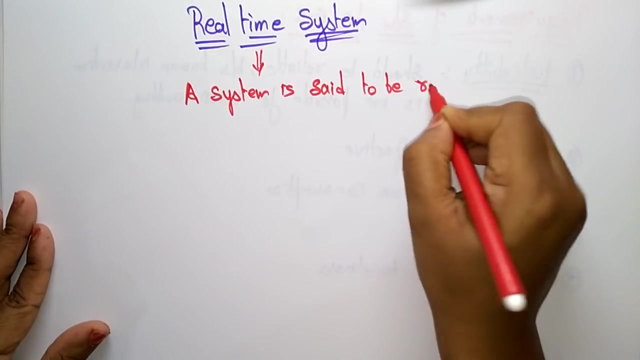 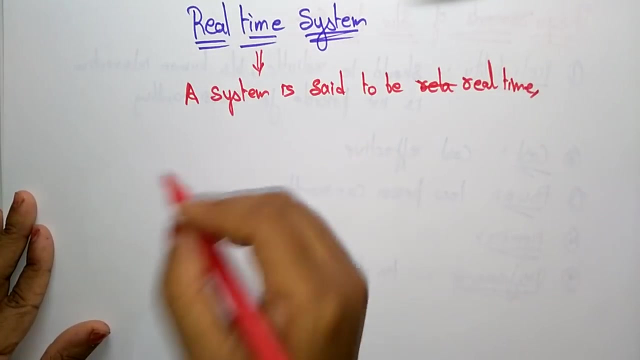 Real-time systems. Okay, So that you are using the technique of real-time systems. So what is this real-time system? A real-time system here? a system is said to be real-time. A system is said to be real-time, Okay, If it is required to complete, if it is. 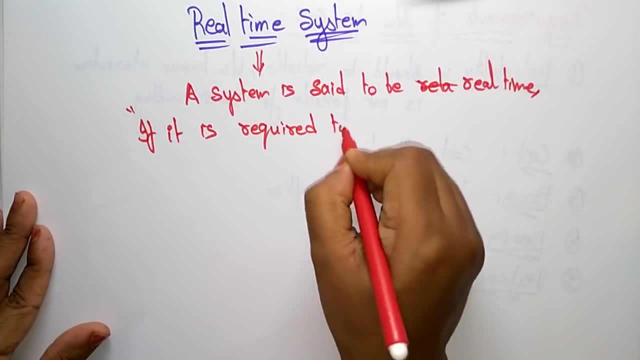 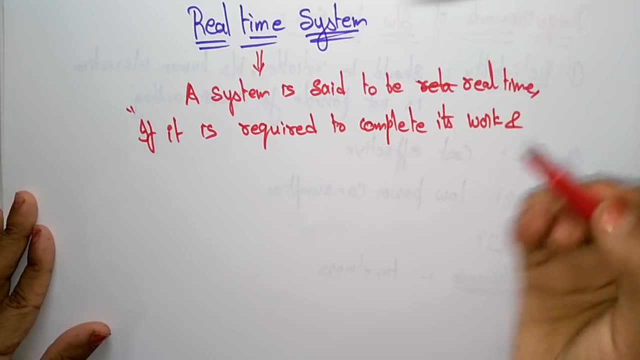 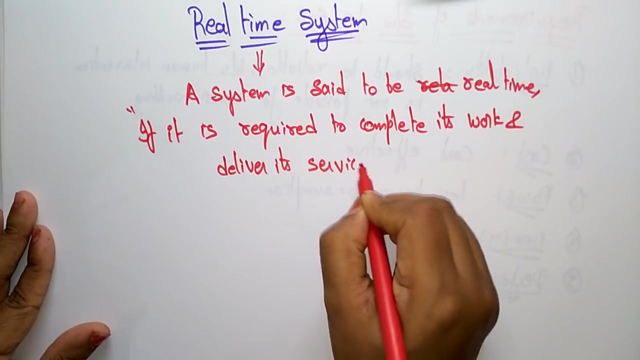 required to complete its work, completes its work and deliver its service on time. and deliver its service services on time, you call it as a real-time system. So whatever the system you are taking, so whenever it completes its work and deliver its service on time, then you can say it is a real-time system. 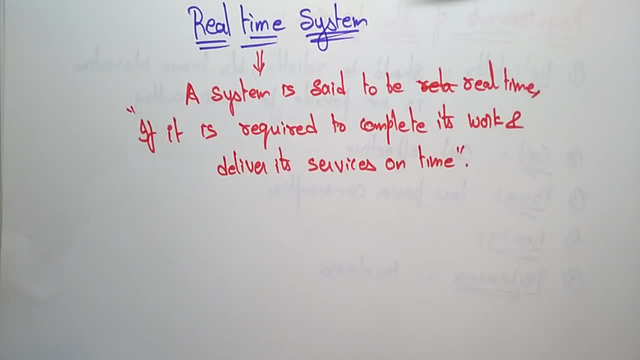 Real-time system. Okay, Suppose, if you are using the mobile, the watch okay, So not sorry the watch you are seeing. okay, the wall clock or hand hand watch something, whatever the watch you are taking, so that watch consisting of some embedded system. 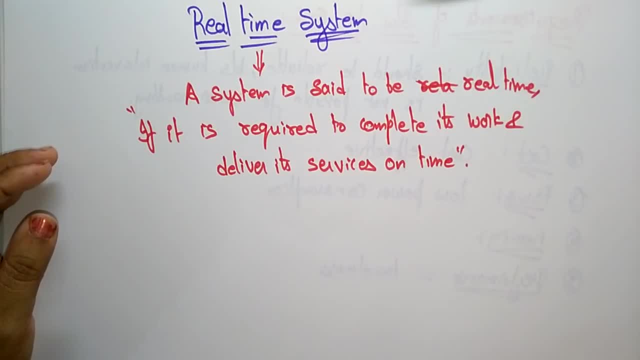 It's a designed hardware as well as a software. So the software is make sure that it is a real-time system. So it is required to complete its work and deliver its service on time. Okay, So any kind of service is required. So it is required to complete its work and deliver its service on time. So any kind of service is required. So any kind of service is required. So any kind of service is required. So any organization should be available to you so that you are the person who can and deliver these services as par in the day. 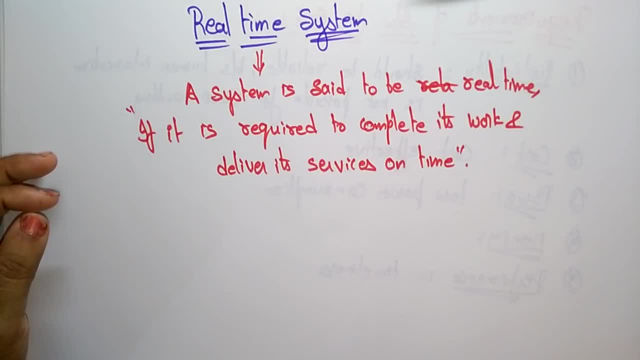 so it's just based on your settings. the time is going to be rotate, okay, so the hands on the clock is going to be rotate. or else you can take the system like oven, micro oven, so you are going to set some time, okay. so just, you want to heat any of the? 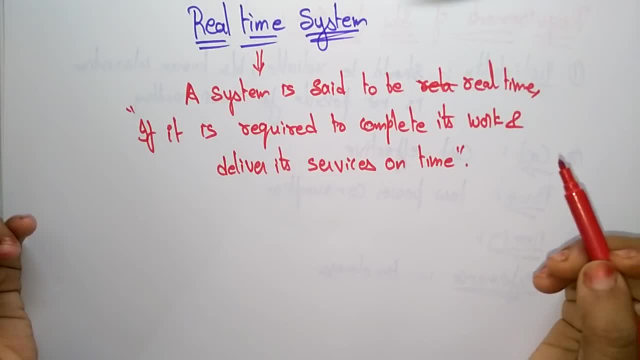 milk or whatever it may be. so just you set the 30 seconds. so here there is a real time system, is there? so here it is going to complete its work and deliver its service on time. so what the time? i set the time as 30 seconds. so within 30 seconds, how much heat it has to be produced? that has to be. 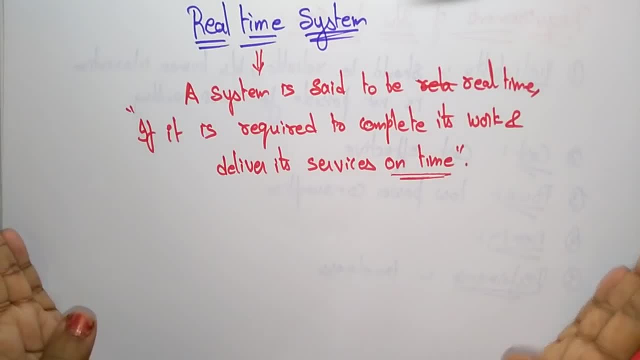 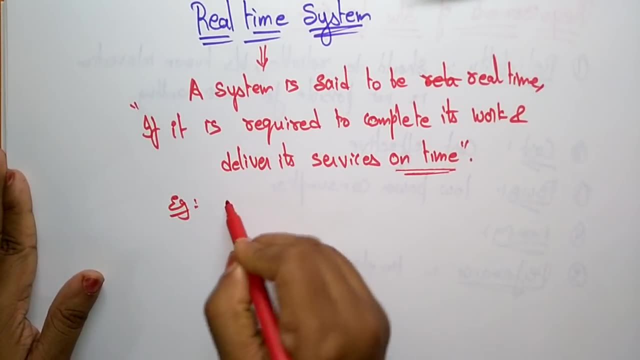 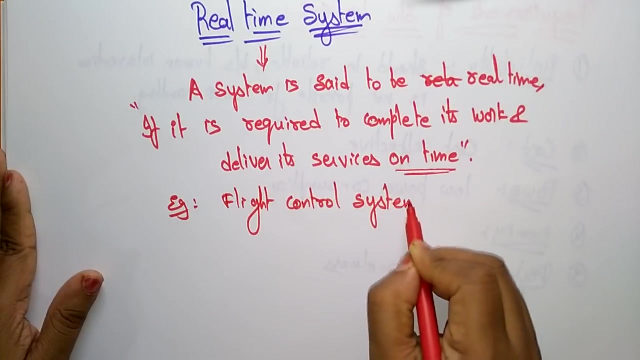 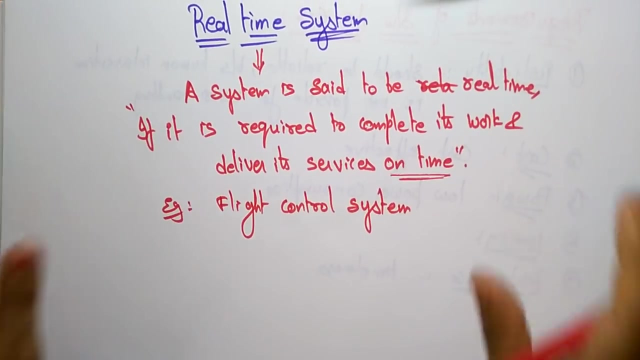 delivered. okay, so that is a real time system. so the real time system is one of the important concept in the mdata system. so let's take the example for this real time system, the flight control system. the time system is said to be, uh, it's nothing, but it is if it is required to complete its work. 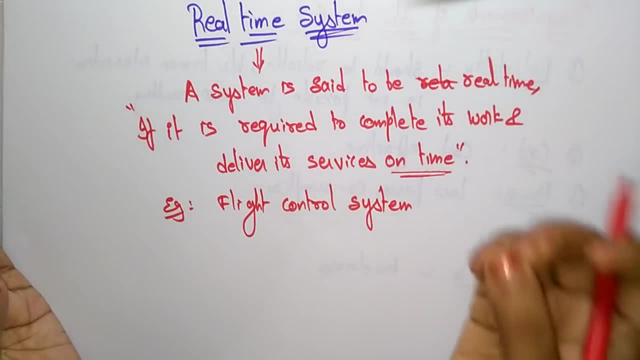 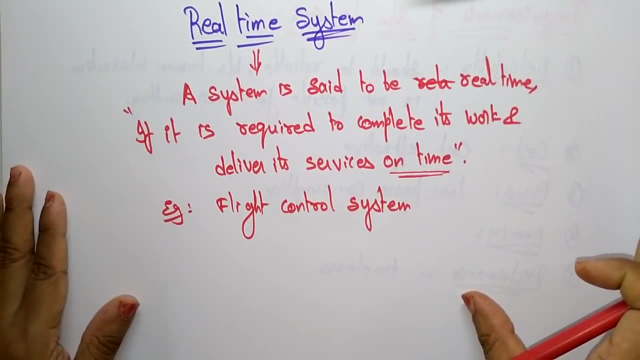 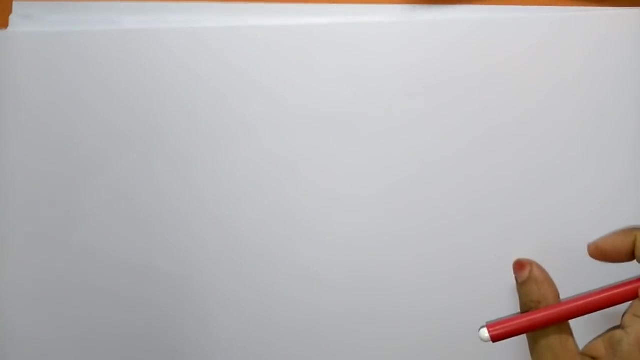 whatever the system, whatever the task you have taken, if that task is required to complete its work and deliver its service on time, then you can say it is a real time system. there are different types of real time systems. so, real time systems, everything will be based on the time constraint. 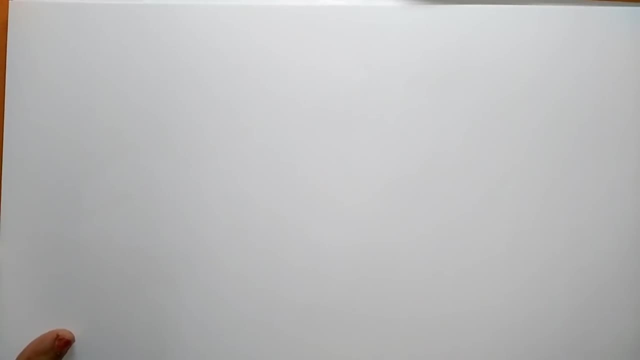 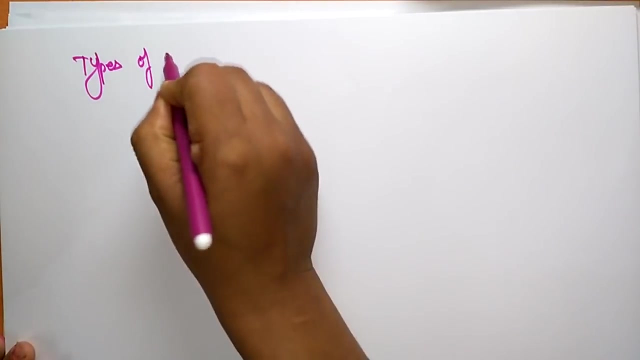 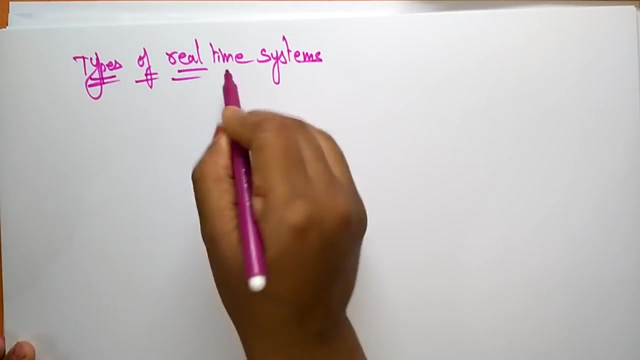 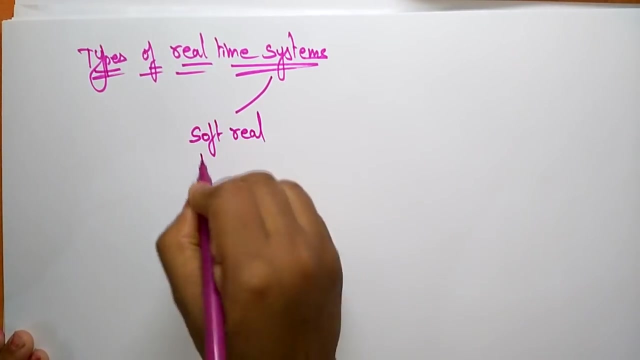 the thing you have to be: remember that it is a time constraints will be. it depends upon time. so, for example, this is one type of flight. so, for example, this is two types of flight. so the lines between these two types of flight are the different types of flight. so, for example, 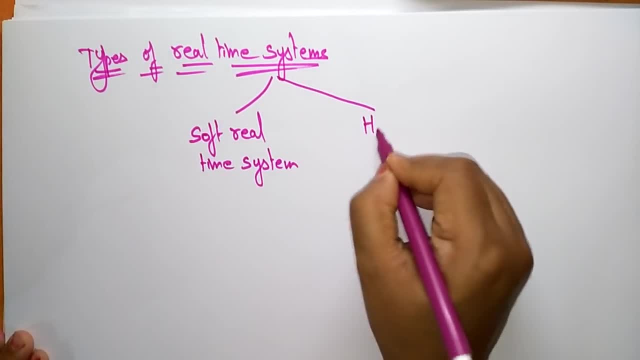 the speed. so here it is. i am indicating the speed because i am indicating the time curve or i am indicating the temperature, and we have consistent of these two types of flight. so let's take a look at this one type of flight. okay, so let's talk about this flight. so first, 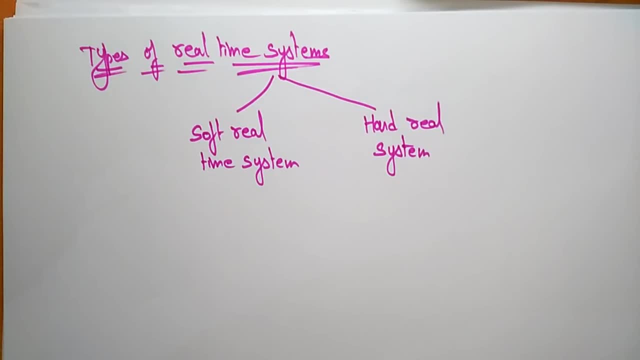 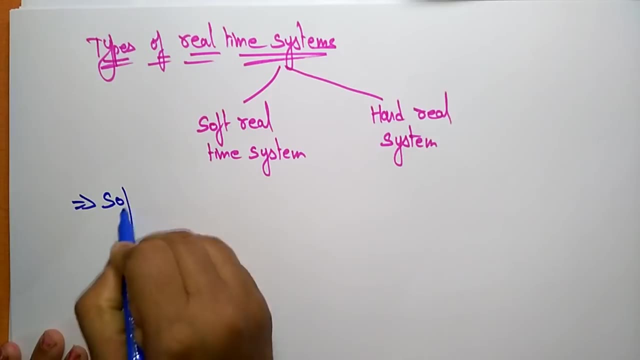 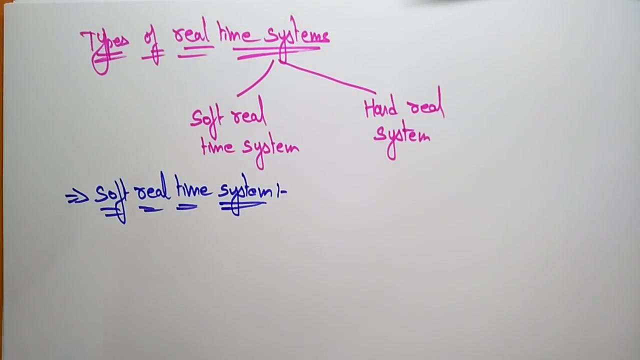 types of real-time systems: soft real-time system and hard real-time system. so let me explain what is a soft real-time system. soft real-time system: so the name is saying that you can work softly. okay, so there is no complete restrictions, or not there in this in the way of soft real-time system. since soft 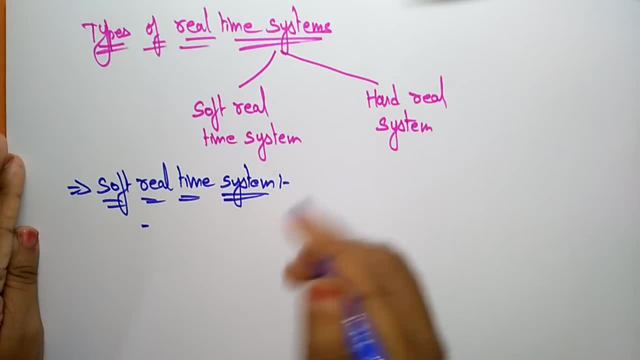 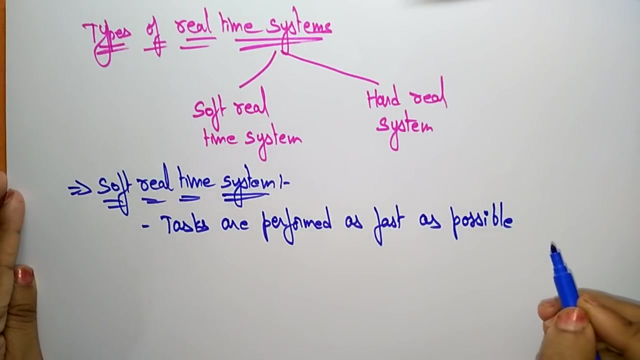 real-time system, tasks are performed as fast as possible. let me write the points: tasks or perform as fast as possible. so late completion of jobs is undesirable but not fatal. so in soft real-time system, so whatever the late completion of jobs will be there, so those jobs will be. 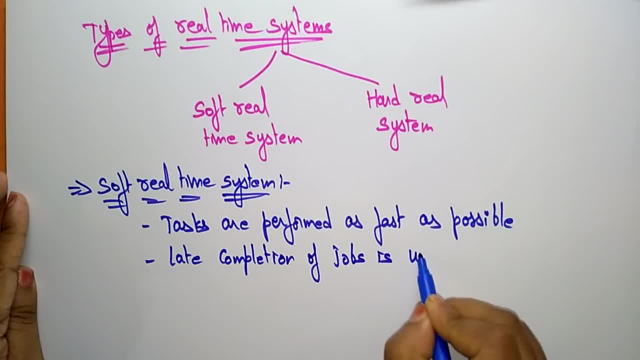 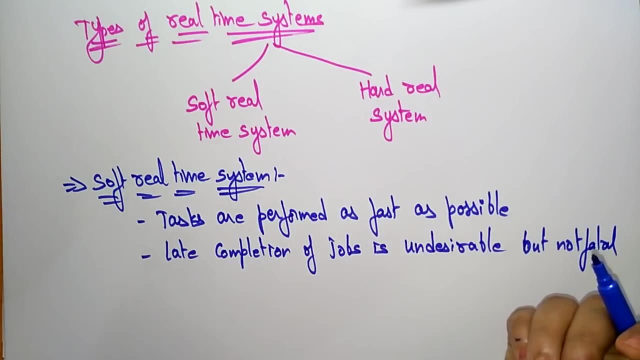 late completion of jobs is undesirable. they are just undesirable, but not fatal. okay, and the system performance degrade as more and more jobs misses the deadlines. so they can, you can miss the job, but when see, you can skip the time also. but if the system, the persistent performance is going to be degraded, if 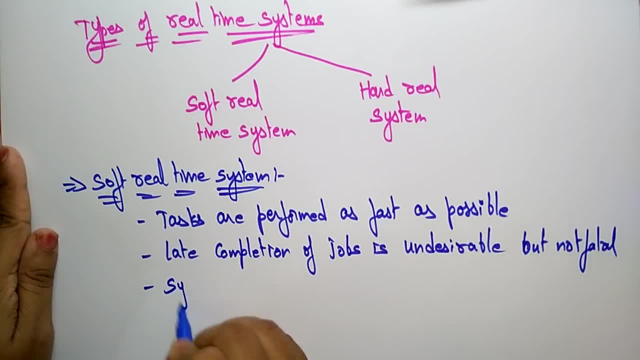 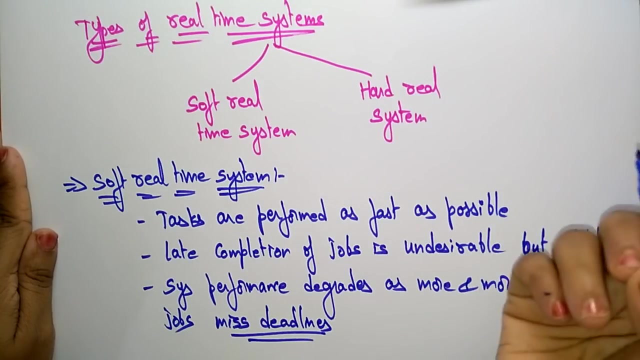 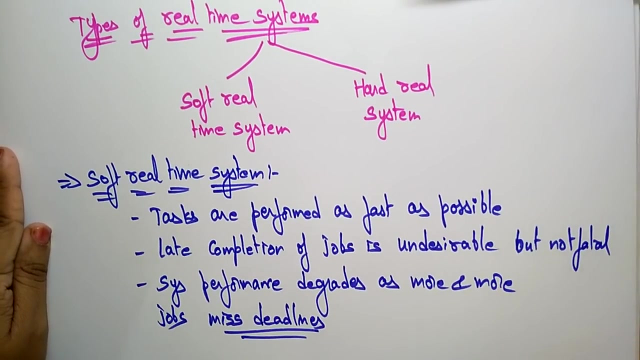 more missed deadlines are there? System performance degrades as more and more jobs are, as more and more jobs miss deadlines. So deadlines means they are given some time. Okay. If that exceeds the deadline, the system performance may be degrade. Means it continuously if it is doing? 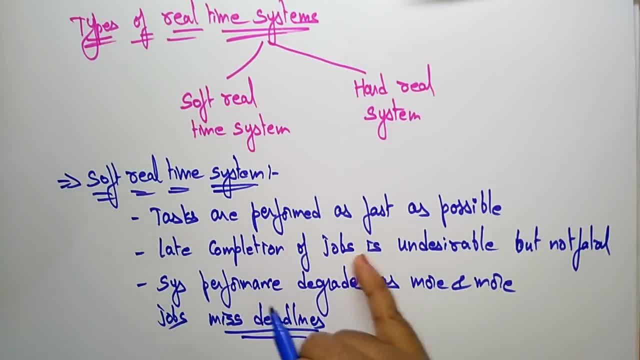 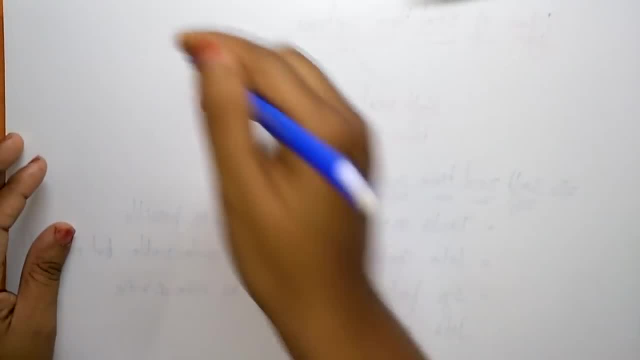 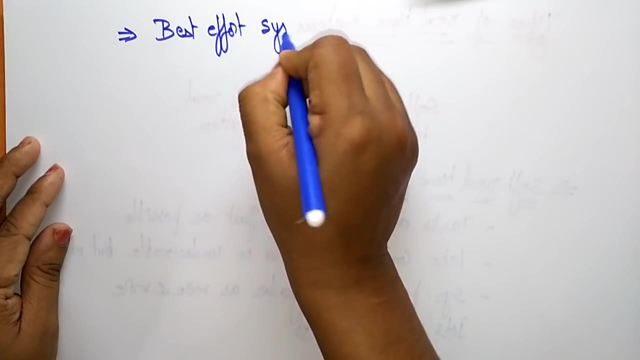 like that, the system performance may be degrade. So late completion of jobs is undesirable, Okay, But not fatal, And it is also known as best effort system, The soft real time system. we can say it is a best effort system, Best effort, We can call it as a best effort system. 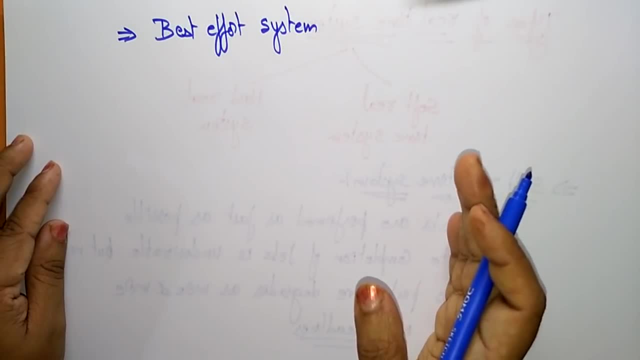 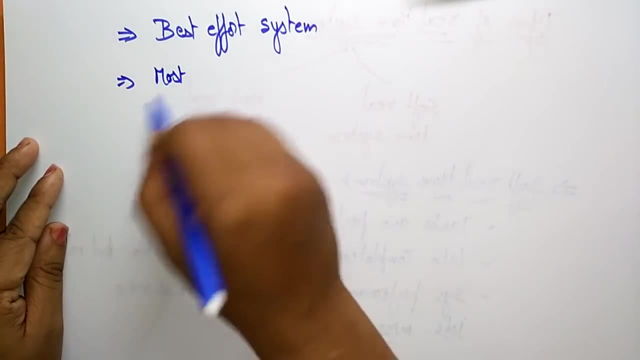 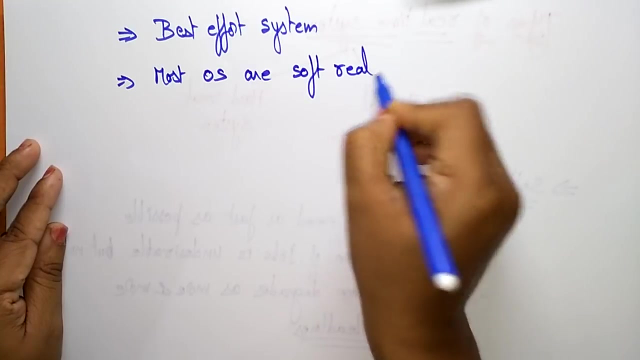 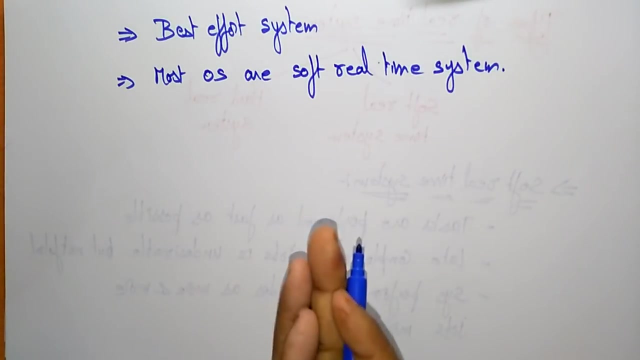 Okay, Most modern operating systems can serve as the base for a soft real time system. So nowadays most of the operating systems are soft real time systems. So the soft real time system means there is no exact constraint, is not there, Okay, So late completion is also you sometimes it is. 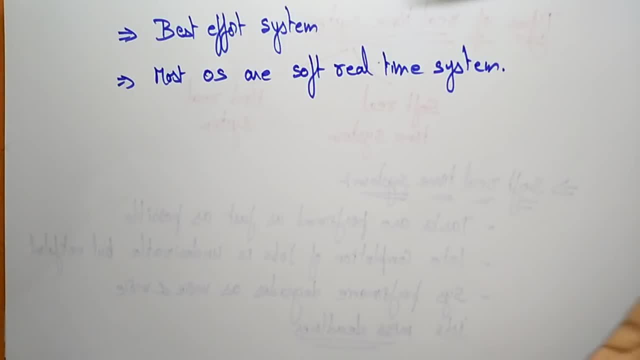 may be possible, or it may be just discard the line, But if the system, if you continue these things, the system performance may be degraded. Okay, If it every time that if the job is misses the deadlines means the system performance may be degraded. So what are the different examples for? 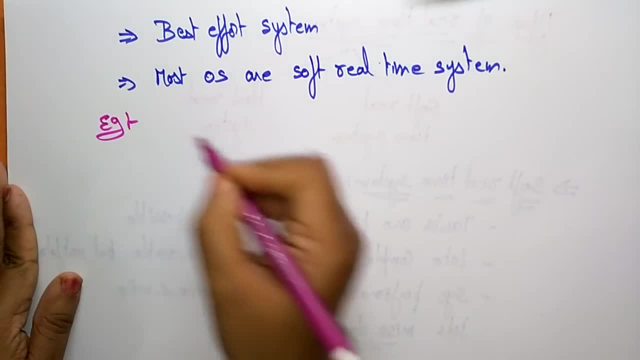 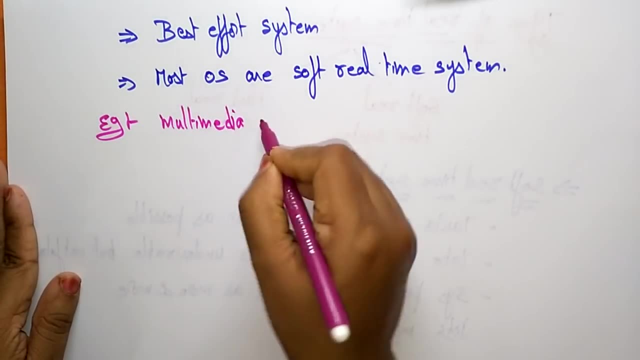 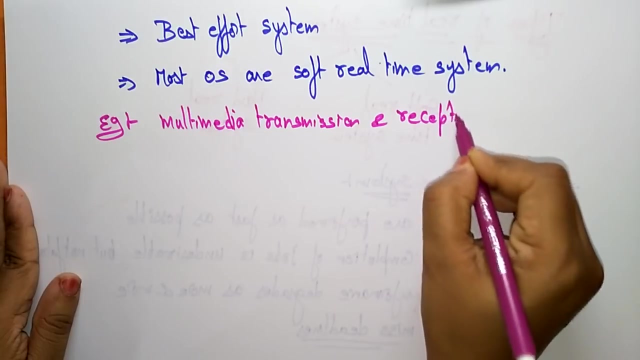 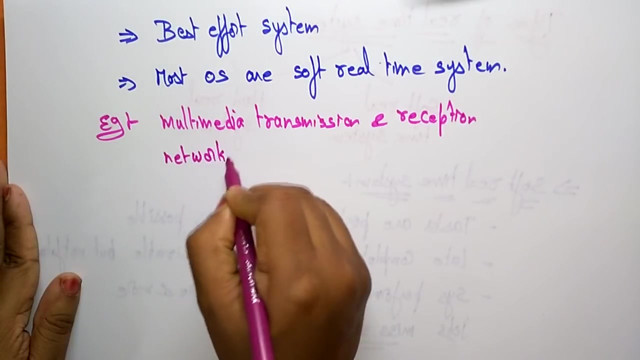 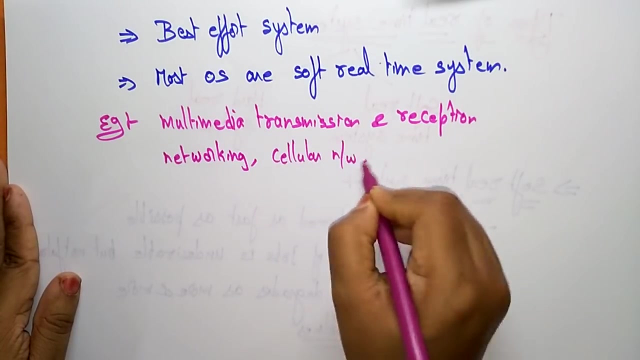 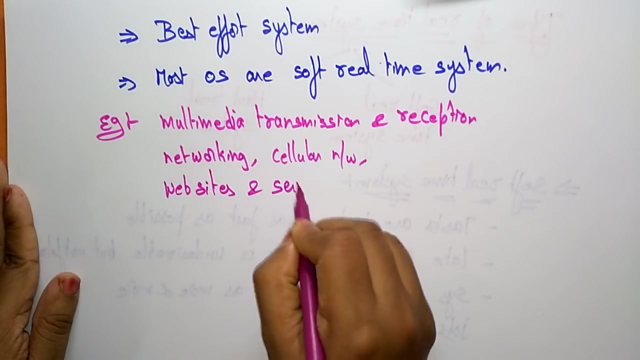 this soft real time system. Let me write the examples: Multimedia transmission and reception, Transmission and receiving, Reception, Networking, networking in telecommunication like cellulars, cellular network and even websites and services, Websites and services. so these are all these soft real time systems. you can say that. 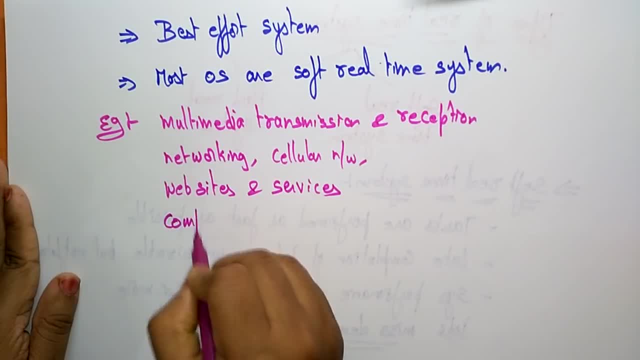 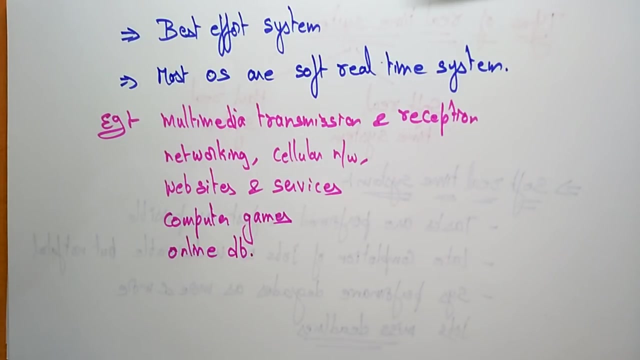 systems and computer games. computer games, online databases. okay, so in online databases also, if you want to retrieve the data somehow, it takes the time but you will get the data. okay, sometime it may not get the data. the page cannot be displayed in the cellular networks. you can sometimes with the, if there is a signal you can able to hear. 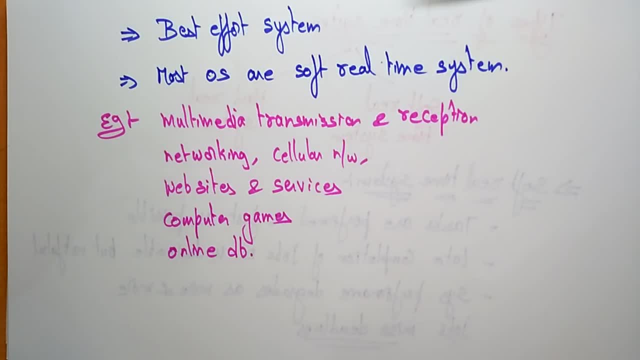 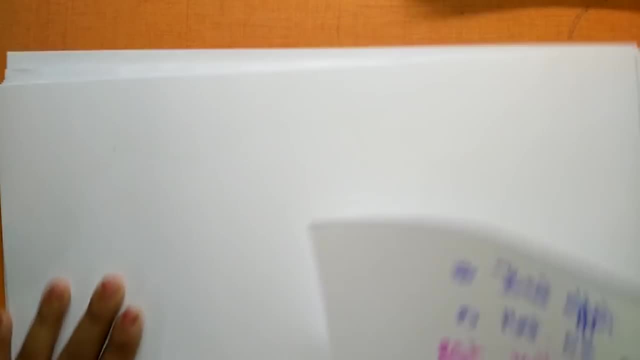 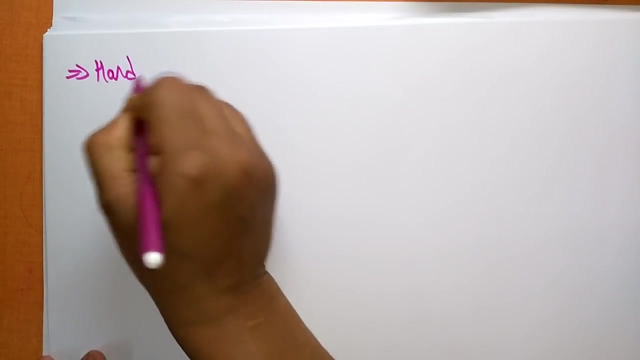 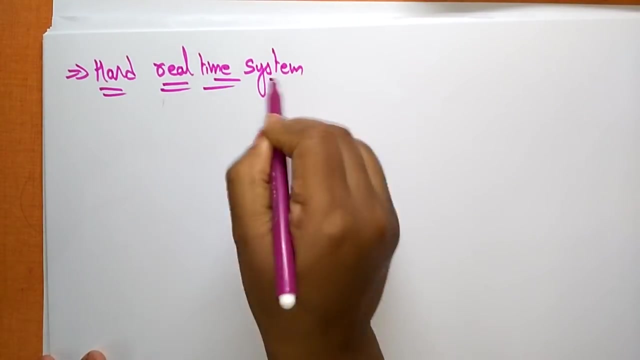 the voice, otherwise you can't hear the voice. sometimes the call may be disconnected. okay, so these are all the soft real-time systems. let me explain the hard real-time system. so what is this hard real-time system? hard real-time system? hard real-time system means there is no. 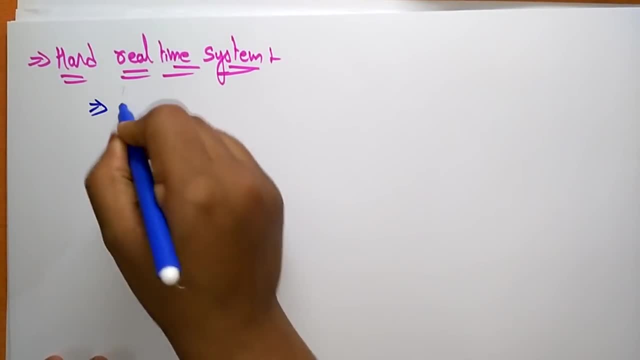 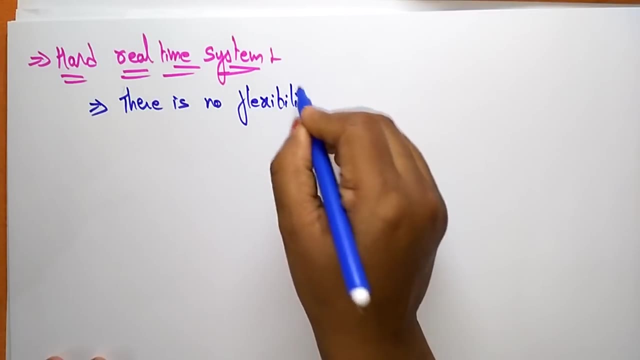 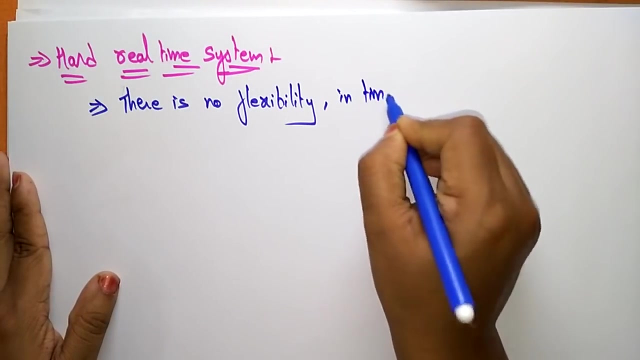 flexibility. so the first thing is in hard real-time system there is no flexibility, just like in the case of soft real-time. but here in hard real-time there is no flexibility, mainly in time constraints. in time constraints, once the time is fixed, means you have to be completed with that work in that time.